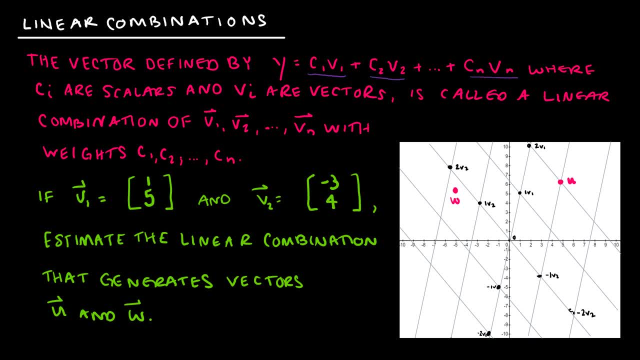 scalar times a vector plus a scalar times a vector, as many times as I need to to generate a new vector. So let's look at vector u and again I've plotted the point u, but vector u would be this line that looks just like that. Now we know from the parallelograms that the vector u is. 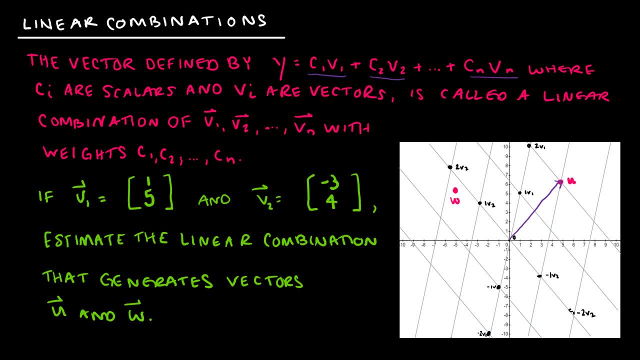 that u would be the opposite corner of a parallelogram. So it's very straightforward for me to draw a parallelogram that looks just like this and I can see, based on that black parallelogram that I've just drawn, that I've got two v1s and negative 1 v2, and so that's how I'm. 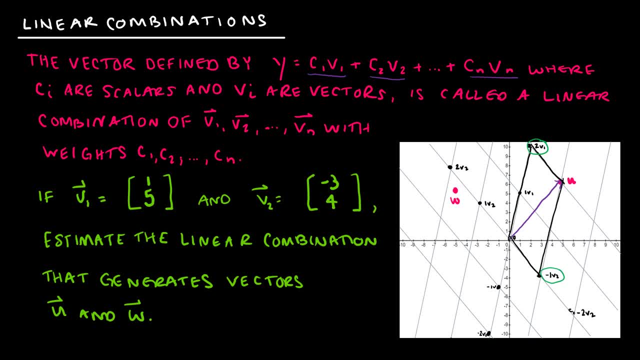 going to draw or write vector u. So vector u would be the opposite corner of a parallelogram. So vector u is generated by taking two v1s plus negative 1 v2.. So I'm going to write minus because it's the same. and that is what vector u would be is two v1s minus v2.. Let's do the same for w. 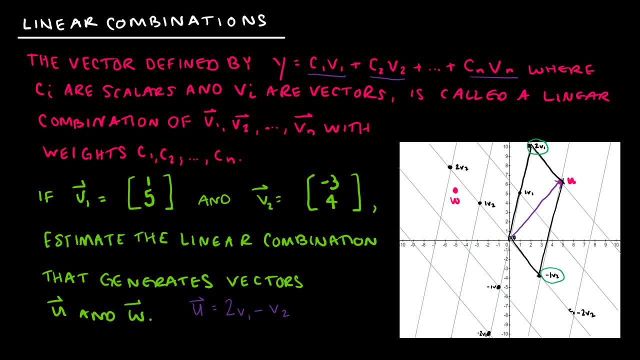 keeping in mind that w is going to be more difficult. So w means that here's my vector and, as you can see, if I try to draw in a parallelogram, I probably should have chosen a color different than black. but we get the idea that I've done a very poor job with this second parallelogram, because w is not the opposite. 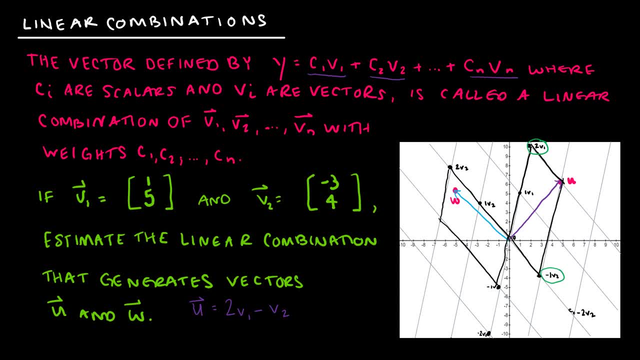 diagonal corner of zero zero. It's just sort of floating in the middle. So let's take a look at how we might fix that. instead, I'll use blue. Use green, because I need it to be different than blue, So it looks like I can go ahead and follow. 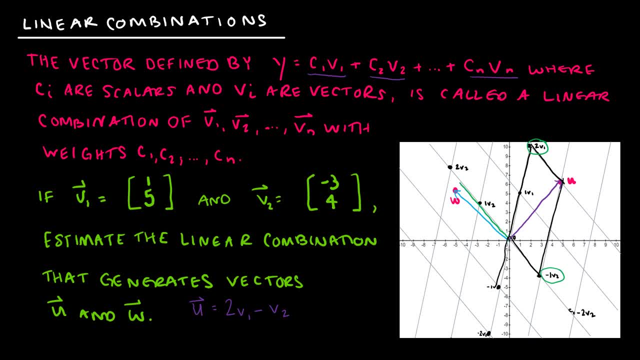 this line and it's going to stop about right here, and I need w to be the opposite corner, which means it's going to look something like this: Now, what does that mean? That means I'm just going to to do some serious estimating. it appears that this might be about one and two. 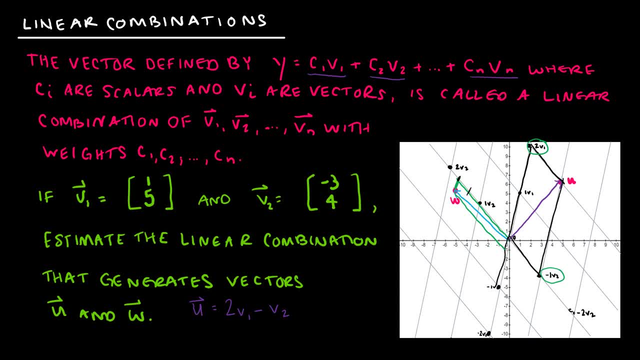 thirds, or five thirds, we'll call it. so vector W is generated by using five thirds of b two, and how many v ones? well, it looks as though it might be a fourth of v one, so one fourth of b1. so that is how I would write: vector w would be one. 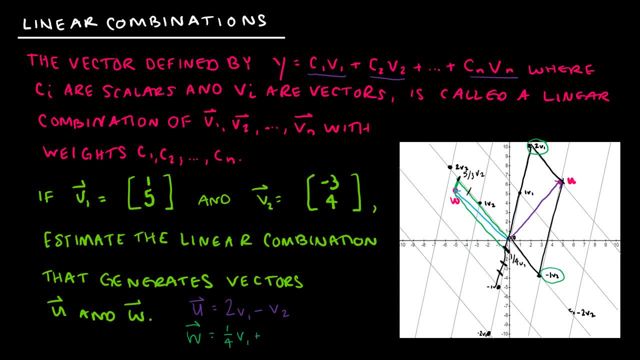 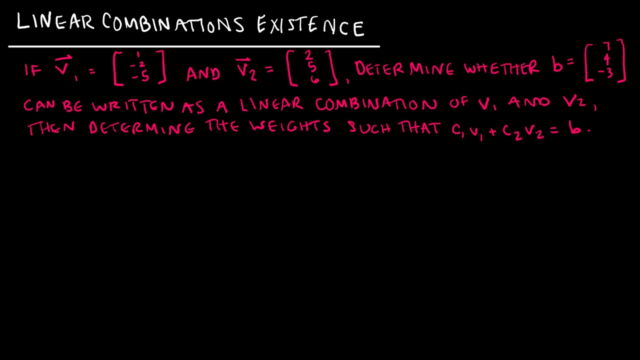 fourth v one plus five, a thirds V 2, and again, that's just an estimation because we're not given anything clear. we've just estimated that W is about a fourth of V 1 and five thirds of V 2. this is a similar question, but it doesn't really look similar. 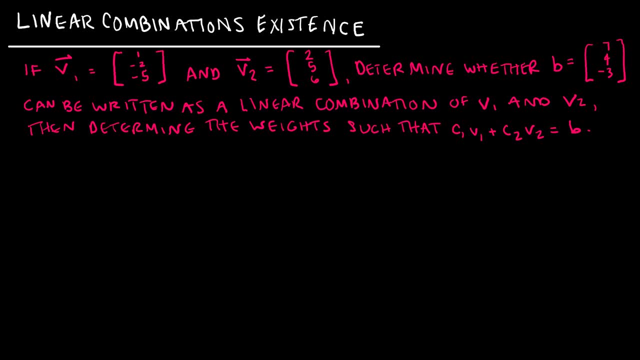 because it's harder. it's harder in two ways. first of all, I can't just draw a picture and connect the dots, so boo, now I have to do actual work. and two, I actually have three values in my column vector instead of just two, so now we're. 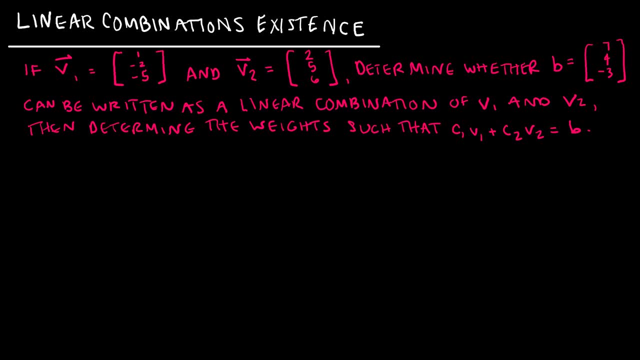 in R 3 instead of R 2, which of course would make drawing a picture much harder and, believe me, you don't want to see me try to draw a picture in three dimensions, so let's go ahead and stick with just the math here. first thing, I 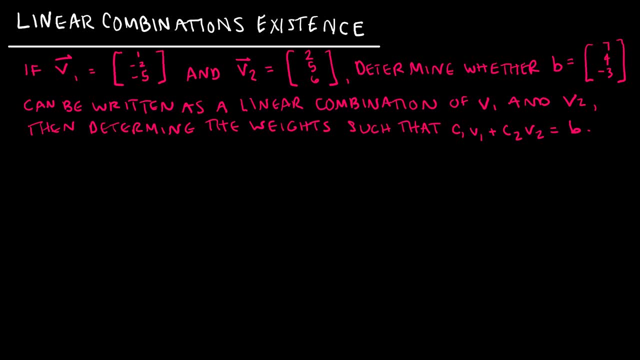 want you to understand is: what is the question asking? it's essentially asking the same thing that our last question asked. it's saying: if I've got V 1 and if I have V 2 and V 3, then what's the question asking? what's the question? 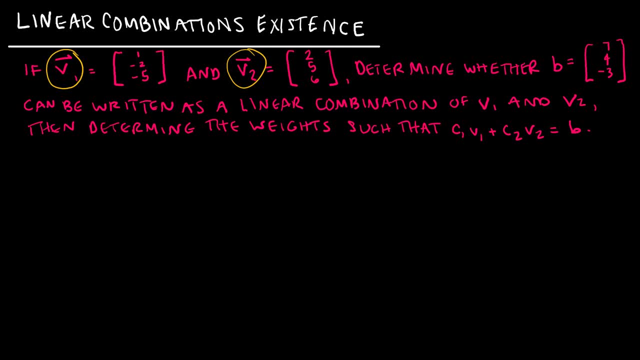 asking. it's saying is we can just use the same thing that we answer V 2? can I draw some sort of linear combination that ends up at 7, 4 negative 3? so in our last examples we just drew a picture. now we have to do math to get us there. so 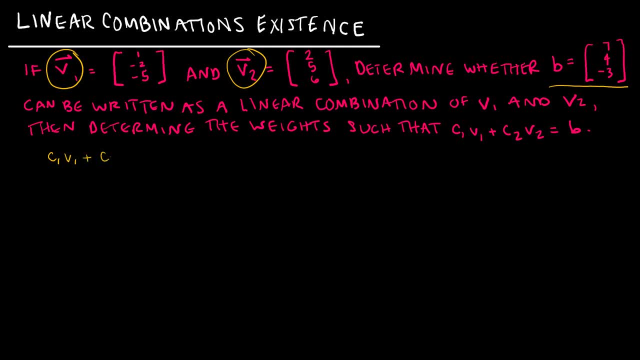 essentially they're saying: is there some C 1 that I can take, times V 1 and some C 2? So let's expand on that. Is there a C1 that I can take times 1, negative 2, negative 5?? 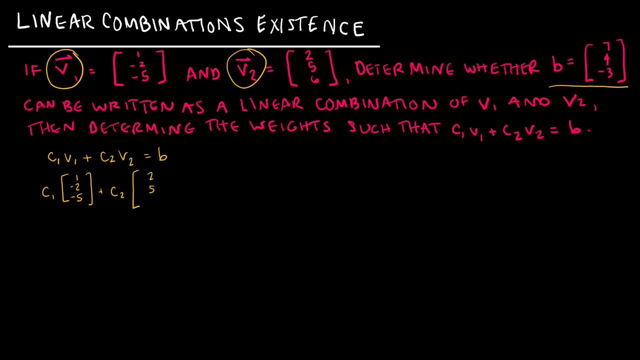 And is there a C2 that I can take times 2,, 5, 6? That's going to end up at 7, 4, negative 3.. Now, if I wanted to- because I know that C1 is a scalar and C2 is a scalar- I could think. 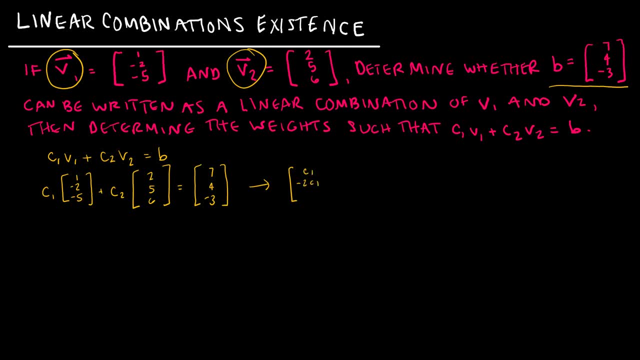 of this as: C1, negative 2C1, negative 5C1 plus 2C2, 5C2, 6C2 equals 7, 4, negative 3.. Now keep in mind that this is just a system of equations and I could write it as: C1 plus. 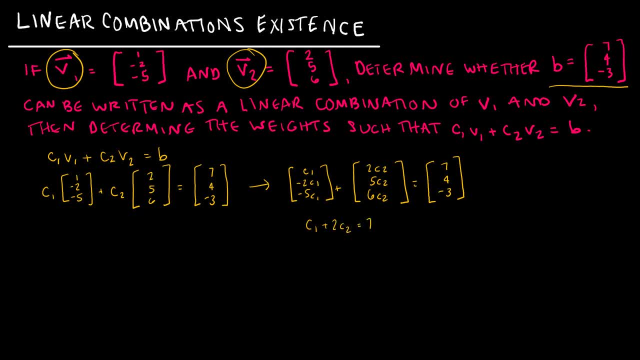 2C2 equals 7. And negative 2C1, et cetera. and I'm not going to do that. And the reason I bring that up is because I know a system of equations can be written as an augmented matrix. 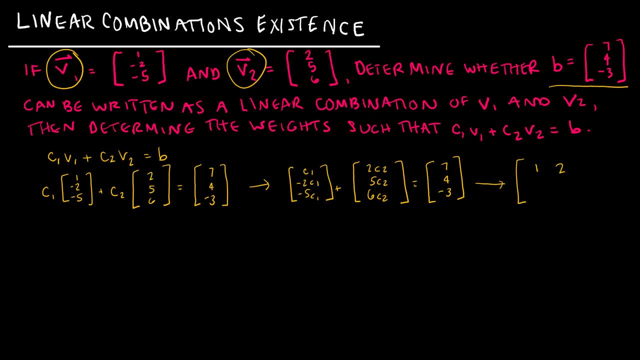 So I'm just going to skip that step and go straight to 1,, 2,, 7.. Negative 2, 5, 4.. Negative 5, 6,, negative 3.. And now I have an augmented matrix. 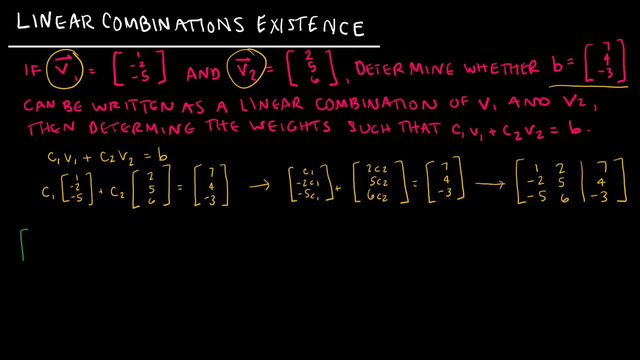 And I know exactly what to do with an augmented matrix. All I have to do is Do all of my magic row operations to end up at reduced row echelon form, and that's going to help me to solve this question. So I've just rewritten the matrix. 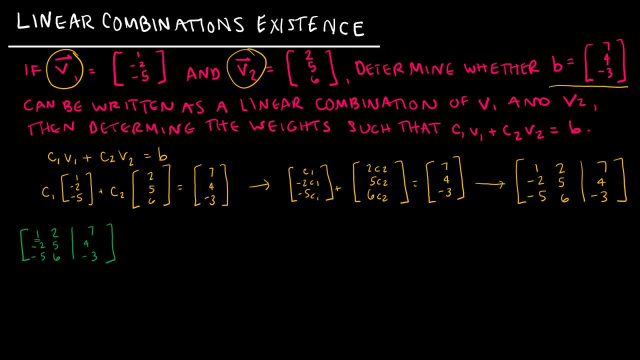 And I've got what looks like a nice pivot there of 1.. And I'm going to make everything below that a 0.. So I'm going to take 2 row 1 plus row 2 to be my new row 2.. 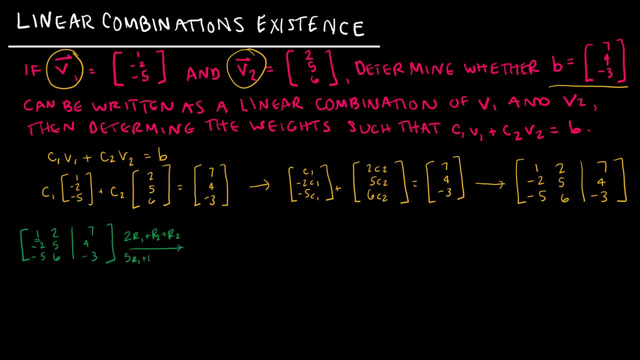 And I'm going to take 5 row 1 plus row 3 to be my new row 3, whoops to be my new row 3.. So that ends up at 1,, 2, 7.. 0, 9,, 18.. 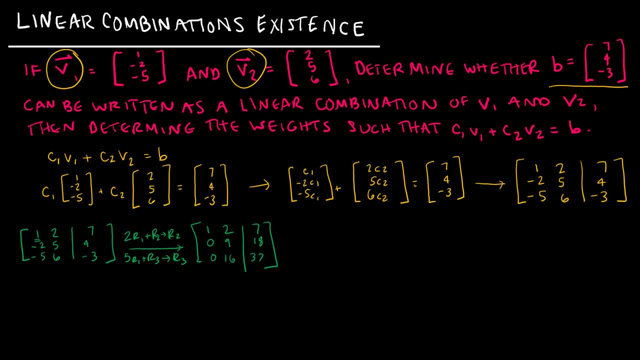 And 0,, 16,, 32.. Now I want that 9 to be a pivot, And I'm going to take 5 row 1 plus row 3 to be my new row 3.. And so I want it to be a 1.. 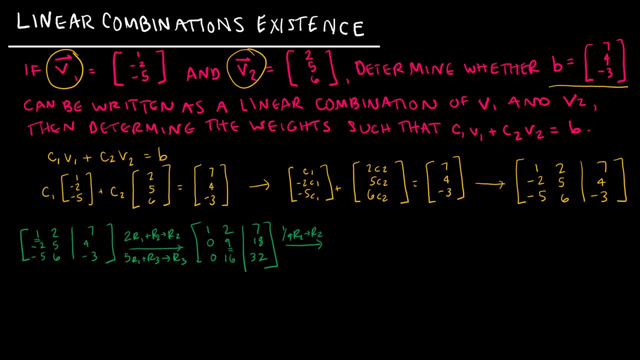 So I'm going to take a 9th of row 2 to be my new row 2.. And that's all I'm going to do in that step. And again, you should be good at row operations by now. So I apologize if I'm going too fast through that, but I don't want to make a 39 minute. 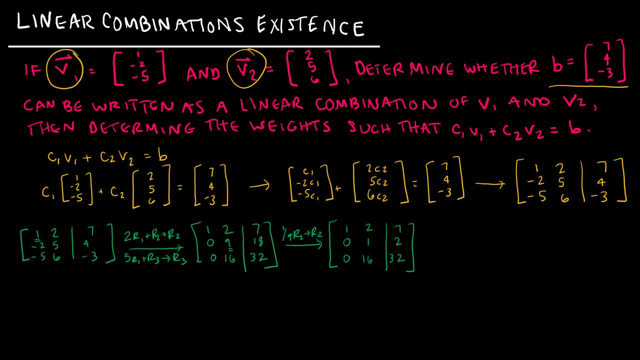 video. I just want to make it as short as I can. So now I have my pivot here of 1, my pivot here of 1.. I want the values above that, I want the values above and below that 1 to be a 0. 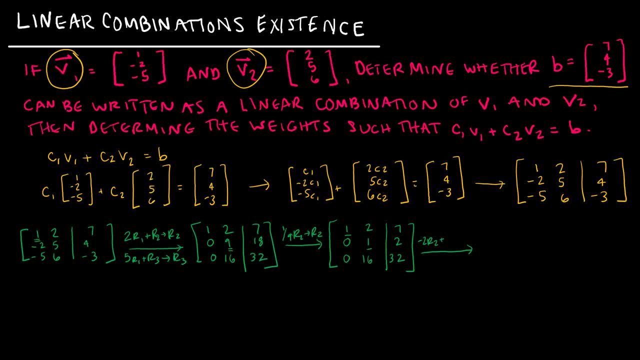 So I'm going to take negative 2 times row 2 plus row 1 to be my new row 1. So that this 2 can become a 0.. And I'm going to take negative 16, row 2 plus row 3, to be my new row 3.. 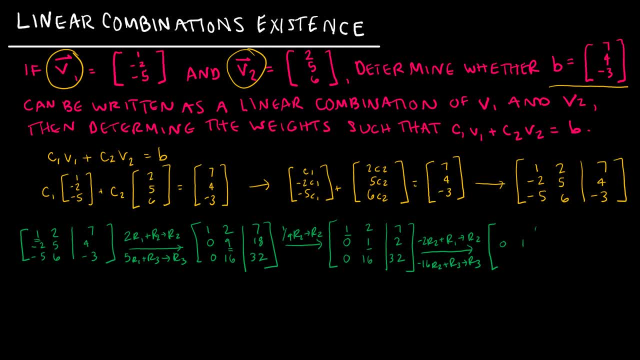 So that's going to give me this guy in the middle. exactly the same as before. My new row 1 is 1. 0. 3.. And my new row 3 is 0. 0. 0.. And I'm fine with that. 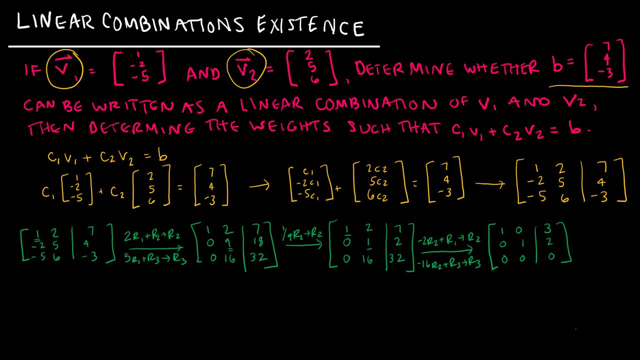 And here's why Keep in mind that this guy is v1 and this guy is v2 and this guy was b. but essentially, what that tells me is what values I'm going to use for c1 and c2.. Because this row says 1C1 equals 3.. 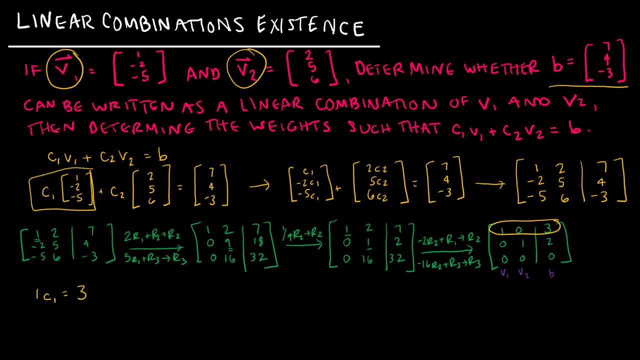 Now again, where did I get that From right? here I've taken C1 times that V1.. So that's what I've done here is I've got 1C1 is equal to 3. And I've got 1C2 is equal to 2.. 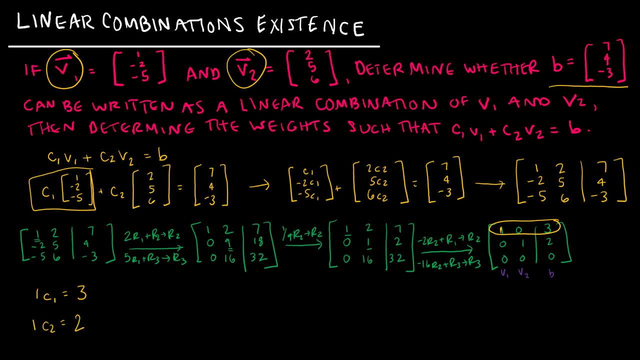 So the question is: can it be written as a linear combination of V1 and V2? Yes. What are the weights? The weights are: C1 is 3, so I could say 3 times 1, negative, 2, negative 5.. 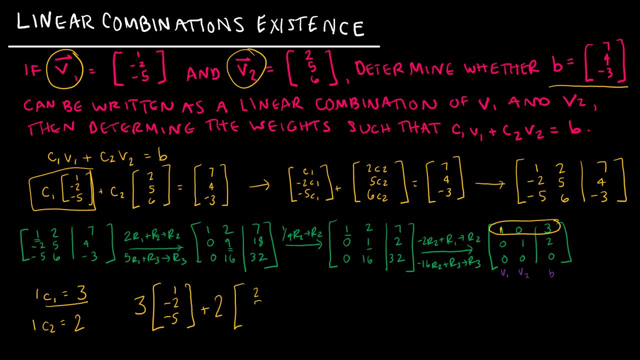 Plus 2 times 2,, 5, 6 is equal to 7,, 4, negative 3.. And again you can very quickly do that mental math In your head to do the check: 3 times 1 is 3.. 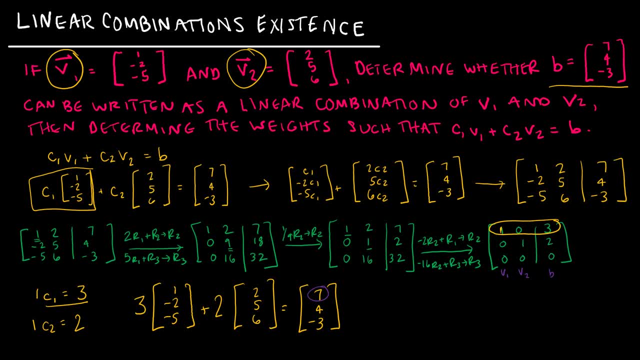 2 times 2 is 4.. Yes, that equals 7.. 3 times negative: 2 is negative 6.. Plus 2 times 5 is 10.. Negative 6 plus 10 does equal 4.. And then 3 times negative 5 is negative 15.. 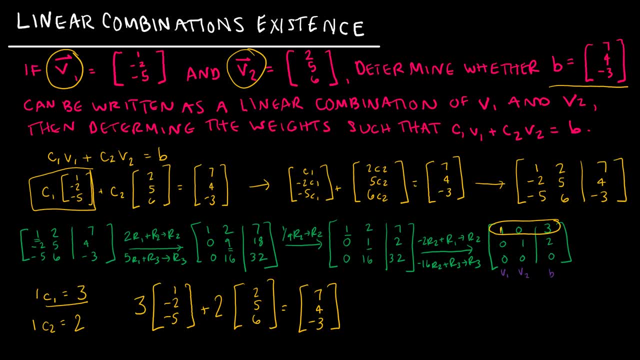 Plus 2 times 6 is 12.. Negative: 15 plus 12 is negative 3. Check, check, It all works out. So again, we've answered this question. We had to do a linear combination. We had to do a little bit more work because we couldn't draw a picture. 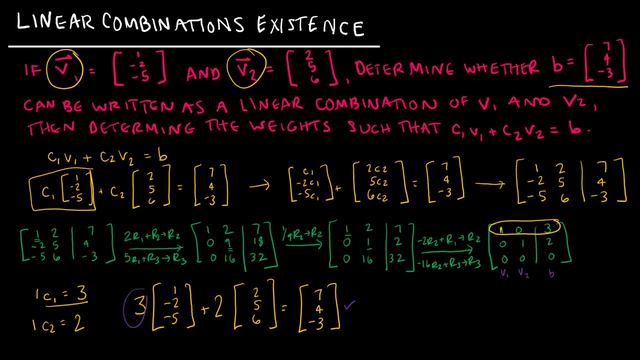 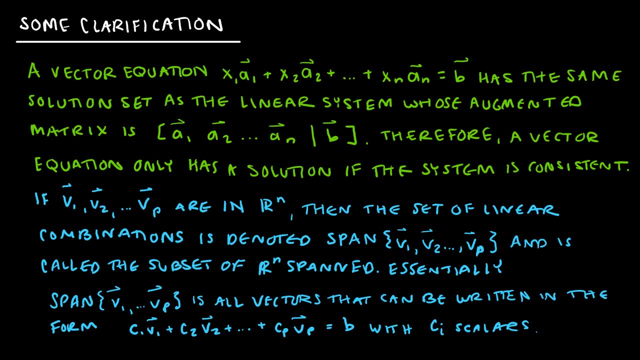 But we were able to answer that question and find the weights of 3 and 2.. So just to drive that point home, or maybe beat a dead horse one or the other, just to clarify a vector equation, which is our vectors multiplied by some scalar, 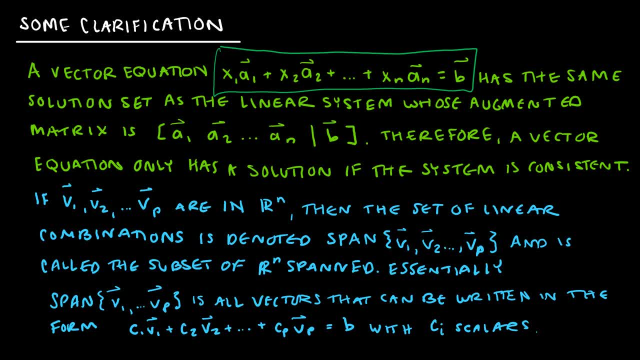 the sum of all of those vectors, multiplied by their scalars, has the same solution, set as a linear system, which is a linear system, which is an augmented matrix, which is a 1,, a 2,, a 3,, etc. 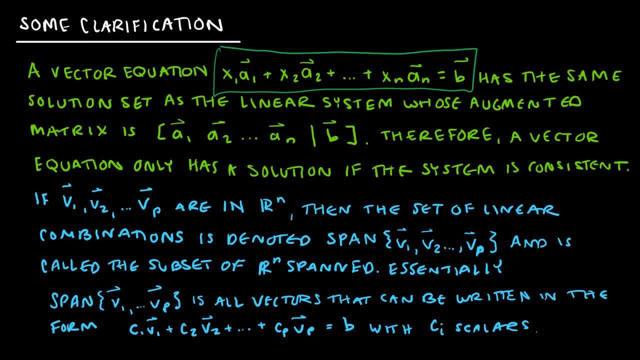 So that is what I tried to make clear on our last example, where I first wrote it as a vector equation and then magically turned it into an augmented matrix and solved that augmented matrix and then magically turned it back into a vector equation so I could see what those scalars were. 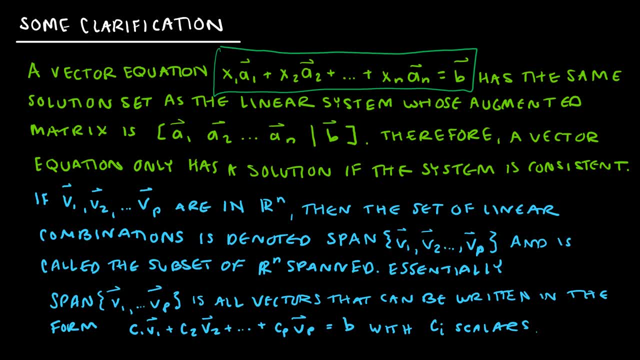 So I just want you to be very clear about the relationship between those things. They're different representations, but they're different representations of the relationship between those things. They're different representations of the exact same thing. I also want to talk about something new. 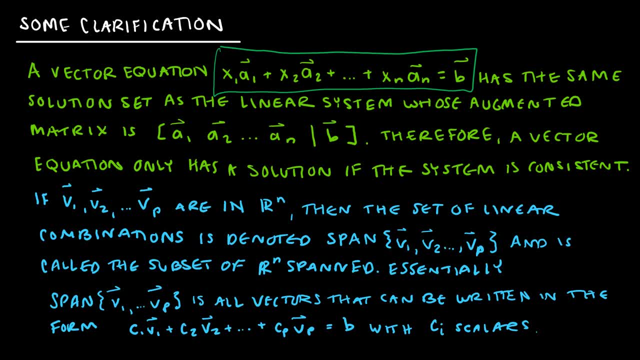 which is a span. So if I have all of these vectors that are in Rn, then the set of linear combinations is denoted span V1,, V2,, V3, etc. and is called the subset of Rn spanned. 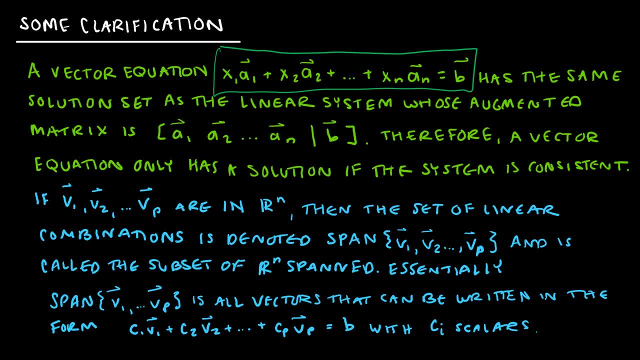 Now you don't see subset of Rn spanned very often but you do see span quite often And span essentially is just the collection of all of the solutions to those linear combinations. So it's all of the scalars. 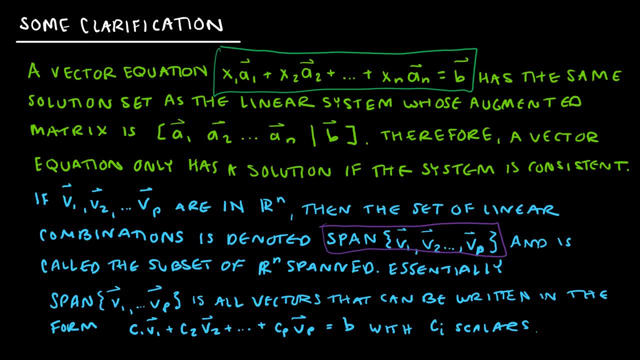 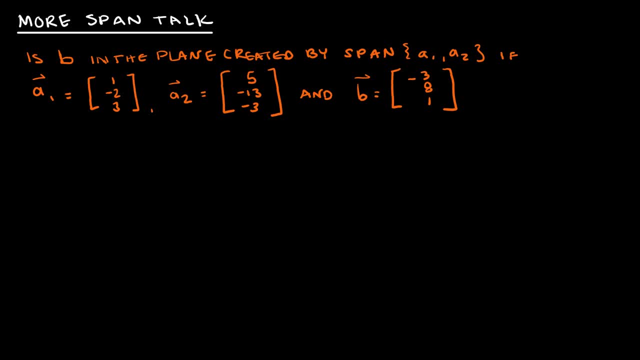 combined with all of those vectors. that are solutions. Now that we know what a span is, let's take a look at this question. It says: is B in the plane created by the span A1, A2? And then it gives us A1, A2, and B. 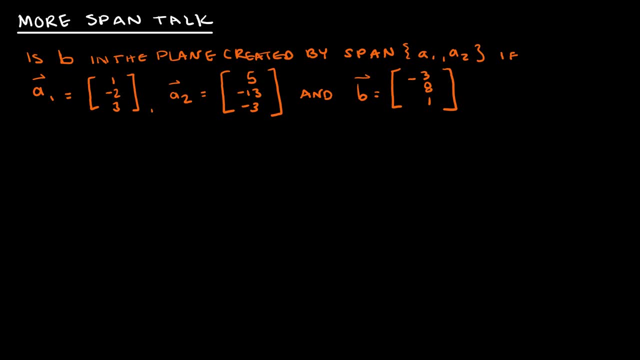 And so this looks like a question that we haven't done before. and yet this is exactly a question that we've done before. Not the same values, but essentially what this is saying is: is there some C1 that I can take? times this matrix, I'm sorry, this vector, and is there some other scalar? 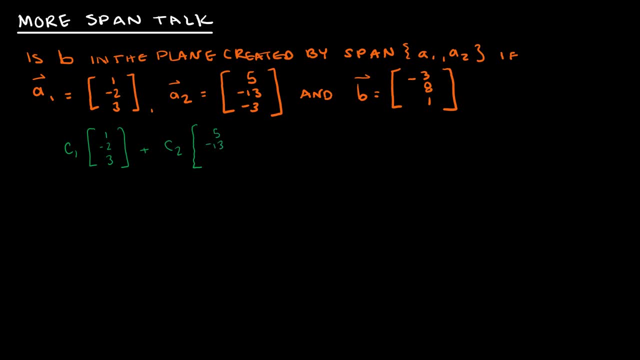 that I can take times this vector that gives me A1? B, And this should look really familiar, because we just did a question exactly like this, And so I'm not going to go through writing this as a system and then turning it into an augmented. 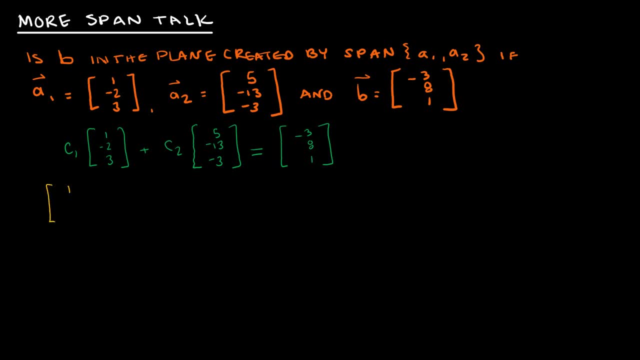 matrix. We're just going to go straight to the augmented matrix. I'm going to say 1, 5, negative 3, negative 2, negative 13,, 8, 3, negative 3,, 1.. And I'm going to say: is B in the plane created by the span A1, A2, A2, and B? 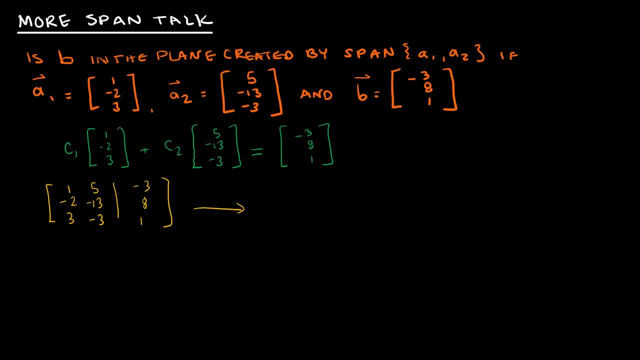 Also I'm going to say is B Au' On my one-dimensional plane Negative 3,, as a remember. so I'm going to try to get this into reduced row echelon form. So let's start by: I've got my pivot of 1 there. let's make everything below it a 0, so 2 row. 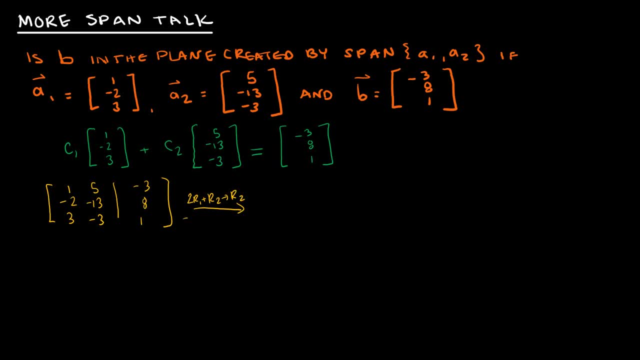 1 plus row 2 is my new row 2.. And negative 3, row 1 plus row 3, is my new row 3.. So row 1 is going to remain the same, and then onto row 3, row 2.. 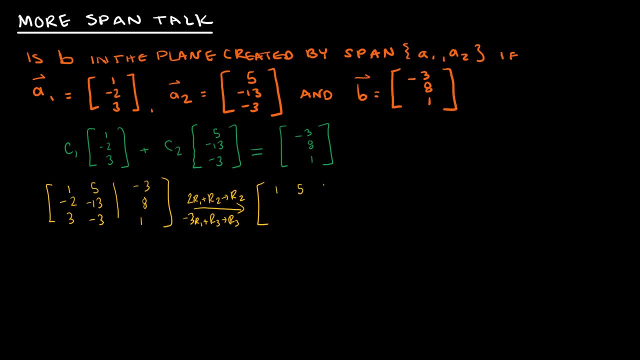 Do a little exploring on my Nat life tree. I had the negotiations form A, the same: 1, 5 negative, 3. row 2. I'm going to end up with 0 negative, 3, 2 and row 3 is going to be 0, negative, 18, 10. now, from here, keep in mind that I want this guy. 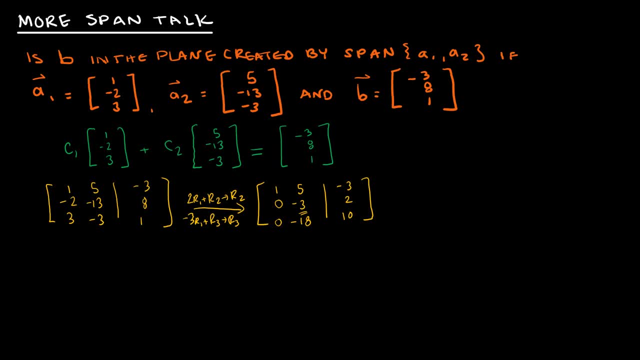 to be a pivot, so I can either divide everything by negative 3 or I can work on getting zeros above and below that. so let's start by just getting a 0 equation, and then this is going to be a row, so I'm going to end up with a row. 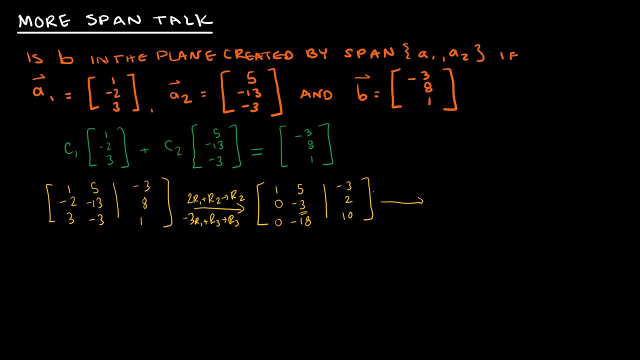 1 and row 3 is going to be 0 negative 18- 10 and row 3 is going to be 0 negative 18 below that. So if I take negative 6 times row 2 and add it to row 3, then I'll get a new row 3. 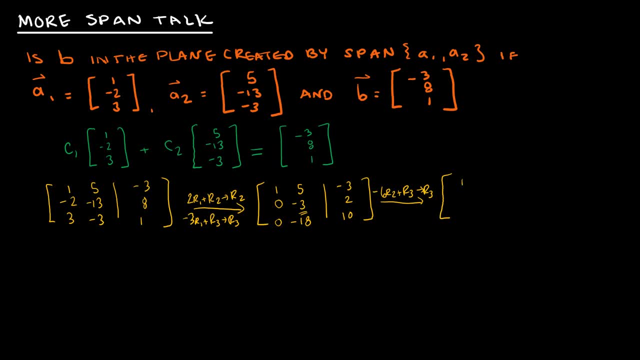 where I've got a 0 where I want it. So this is still going to be 1, 5, negative 3, and this is still going to be 0, negative 3, 2, and this is going to be 0 and 0,. 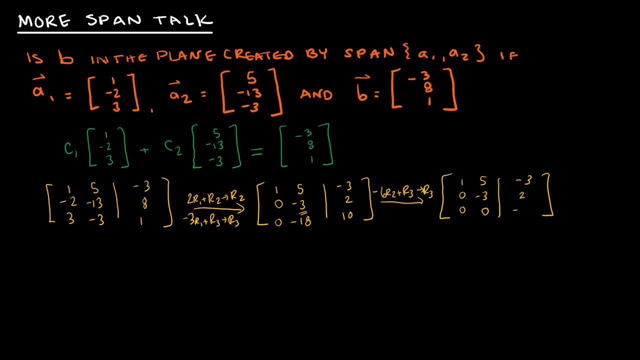 and I get negative 12 plus 10,, which is negative 2, and here's where we have an issue, Because remember what this is saying is that 0 equals negative 2, which, of course, is not ever going to be the case. So this essentially tells us that this vector equation has no solution. 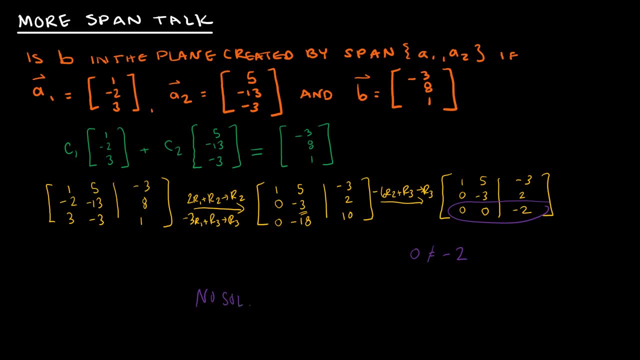 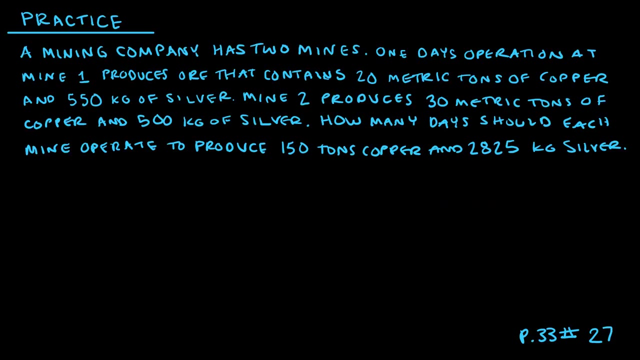 So that b is not in the span a1, a2.. So it says: is b in this plane created by span? and that is of course the answer is no. Here's a practice for you and this is an application question. obviously I haven't already put this into the vector equation for you. 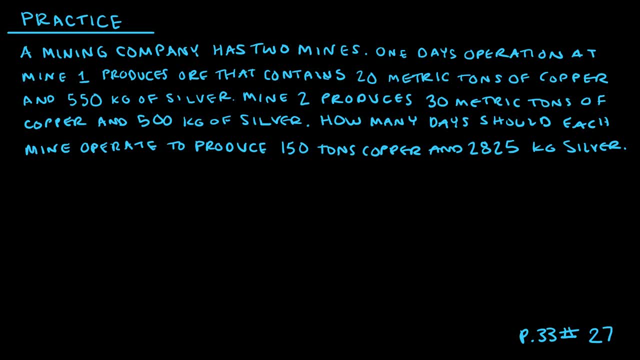 so I'm actually asking you to write the vector equation first and then use that to write the augmented matrix and solve. So if you would press pause, read through the question and then solve, So again what we're being asked to do here. 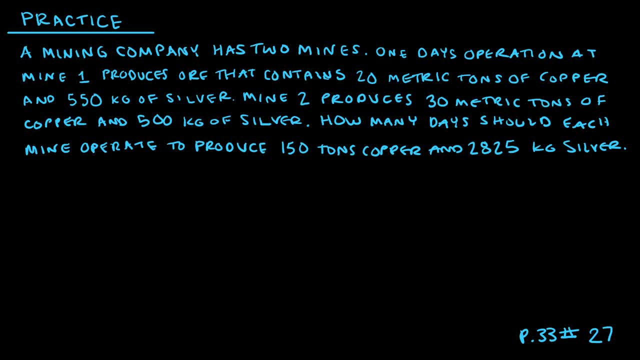 is, we have two mines and we're saying: how many days should I operate mine 1, where I have 20 metric tons of copper and 550 kilograms of silver every day, and how many days should I operate mine 2, that has 30 metric tons of copper and 500 kilograms of silver every day, so that I end up with 150 tons of copper and 2,825 kilograms of silver? 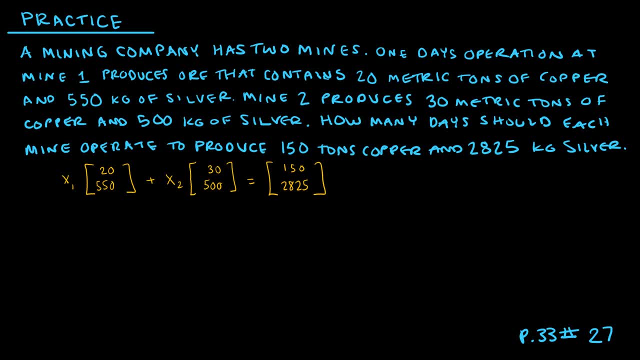 This is the question being asked Now: how do I solve this? Hopefully, we're very comfortable with this at this point. I'm going to turn this into an augmented matrix and I'm going to use my row operator And I'm going to use my ray-or-ray to 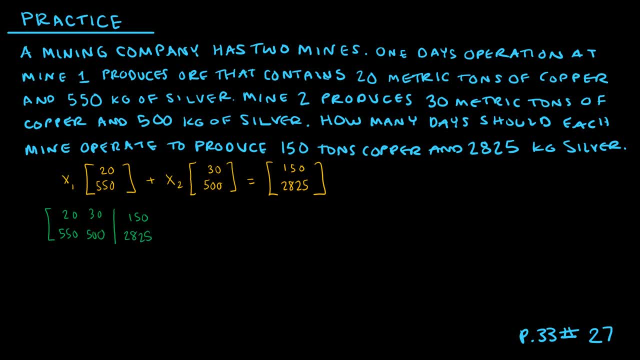 try to say, Cecin, can you reach this? and then I'm going to take my number of Public and then I'm going to take the number of operations. Oops, Yep, that's right: 528, 25.. And I'm going to solve it. 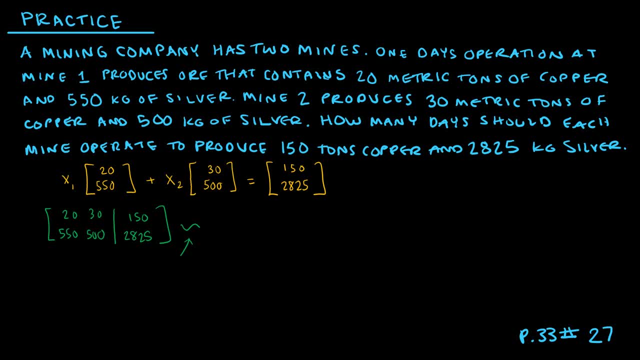 So, for the sake of time, I'm going to use this notation Now. this notation just means that the matrices are equivalent, So I'm not going to show you each row operation this time, but I am going to show you the results after each row operation. 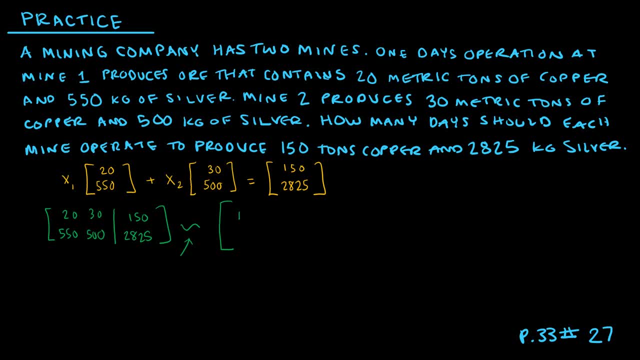 first row by 1, 20th, which gives me 1, 1.5, 7.5 and row 2 I haven't done anything to yet, and now that 1 is a pivot, I need to make 550 into a 0, and so what I'm going to do is take. 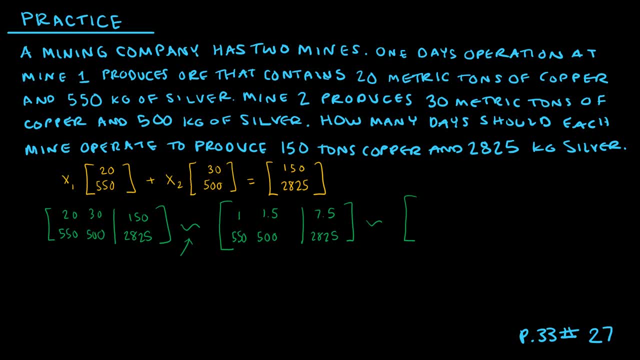 negative 550 times 1 times row 1 and add it to row 2 to get my new row 2. so whoops, this is still 1, 1.5, 7.5 and this guy is now 0, negative 325 and negative 1300. 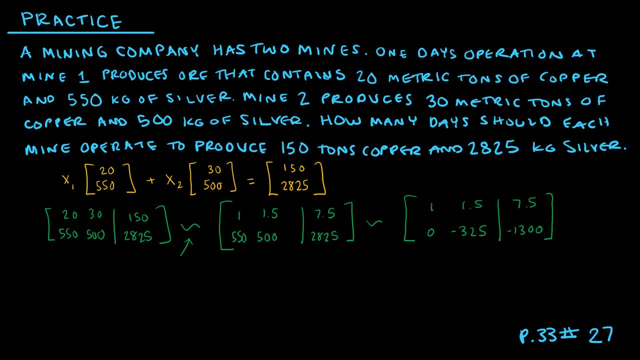 and again that's negative 550 times row 1 plus row 2. so row 1 is looking kind of good, but row 2 is not quite there yet. row 1 is going to remain the same and I'm going to make 550 into a 0, and so what I'm going to do is take negative 550 times row 1 and 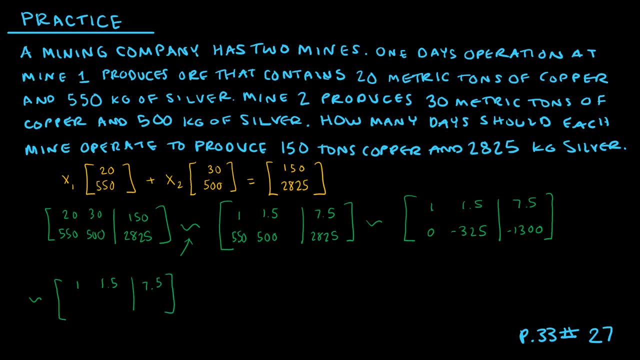 I'm going to take everything in row 2 times negative 1 over 325, which gives me 0 here, 1 here and 4 here. and so now I've got this pivot right where I want it, but above that I want it to be a 0. so I'm going to take negative 1.5 times row 2 and add it to row 1, giving me 1, 0, 1.5. 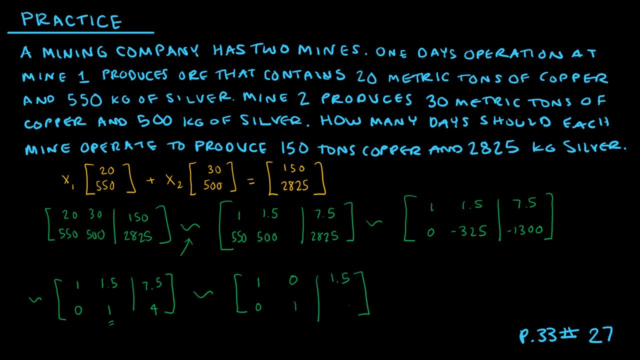 and 0, 1, 4. so the question says: how many days should we operate each mine so that we have the correct amount of copper and silver? and my answer is right here. so I would operate mine 1, 1.5 days and mine 2, 4 days in order to have the required amount of copper and silver. so I'm going to take 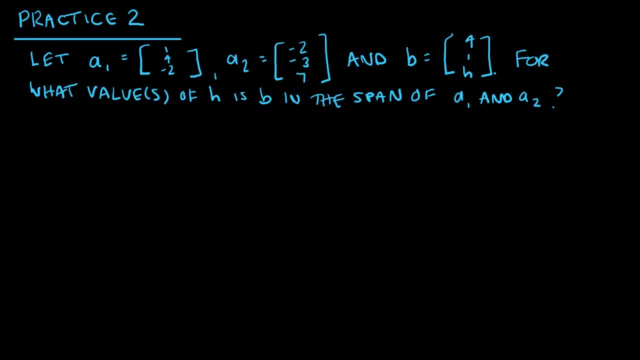 negative 1 times row 1 and enter it into this here, because I have a charge here. I'm going to take negative 1 times row 3 and add it to row 4 into the box and I'm going to have the correct amount of copper and silver. so that's a previous question. I haven't gotten through with you. we've. 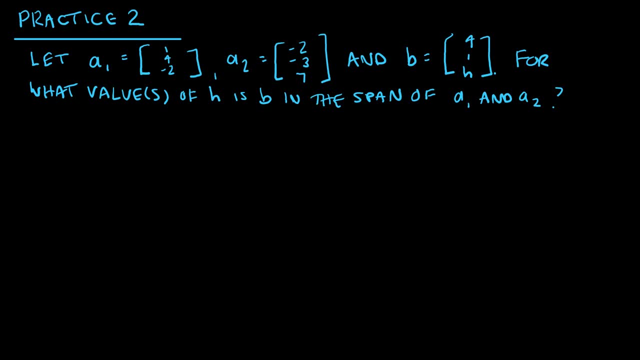 done a similar question in a previous video, but essentially I'm asking a similar question to what you've just done, but I'm asking for what value of H? for what value or values of H is b in the span of a 1 and a 2? so we see this word again, span, which of course means that I'm going. 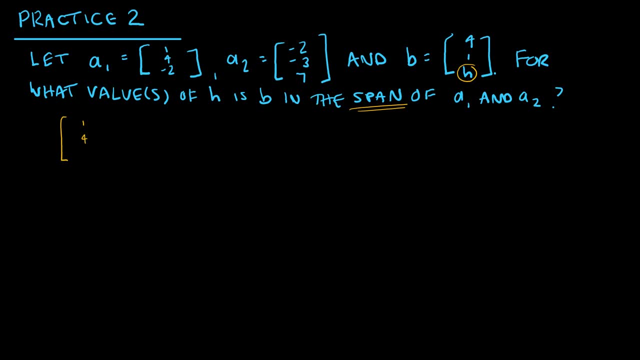 augmented matrix and the question is: can I find the value for H to make this work? so I'm going to leave you there for just a moment. if you would press pause, go ahead and see if you can finish this question and answer for what value or values of H would be be in the span. if you're totally stumped, you can just wait. 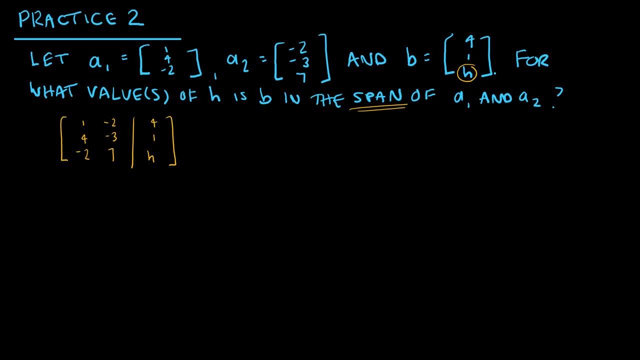 for me to go through it. otherwise, I would like you to try it on your own when you're ready. press play to see how you did so. again, I'm going to use this abbreviated notation and just tell you what the row operations are. my first row is going to remain exactly the same. my second row, I'm going to take negative 4. 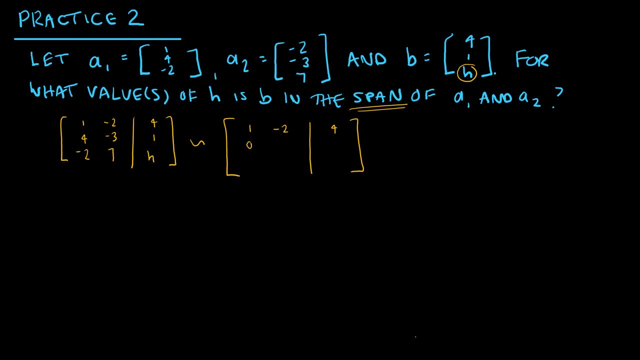 times row 1 plus row 2, so that's going to give me a 0 here, it's going to give me a 5 here and it's going to give me a negative 15 here, and I also want a 0 where my negative 2 is. so I'm going to take 2 times row 1 plus. 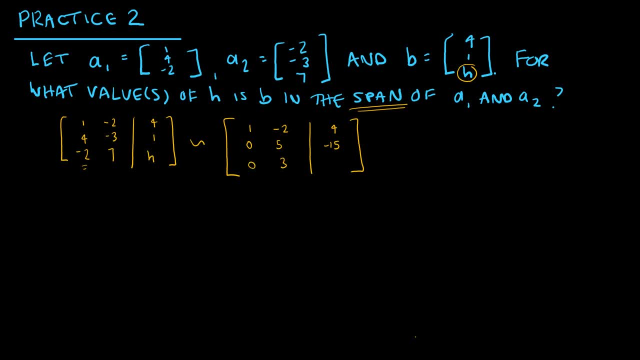 row 3, which gives me 0, 3 and 8 plus H. so far, so good. now, of course, that one was my pivot. I want to make this 5 a pivot, so I'm going to take just a fifth of row 2 and that's the only thing I'm going to. 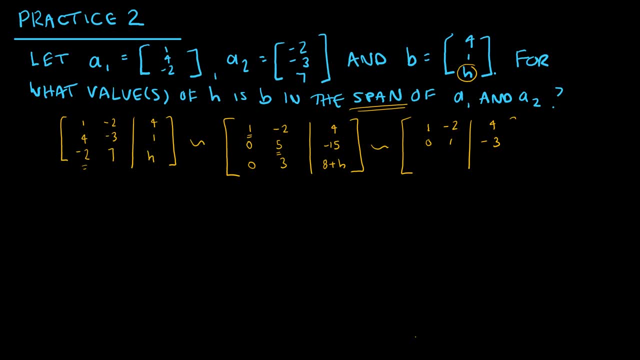 do on this step. so that's 0, 1, negative 3 and this guy remains the same. now, because this- and this is a pivot- I want everything below 1 to be a 0, so I'm going to take negative 3 times row 2 to be and add it to row 3, so that's going. 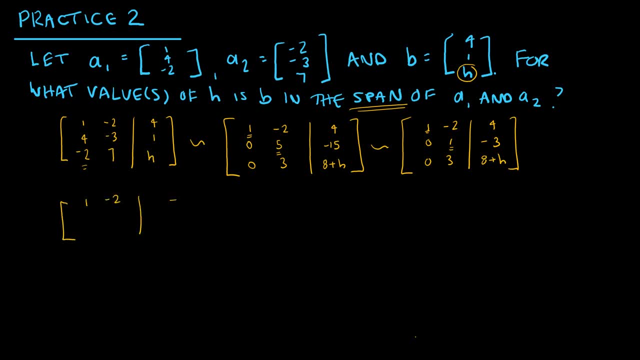 to give me the same row 1. 2 is going to remain the same as well, and I'm taking negative 3 times row 2 to add it to row 3, so that gives me 0 here and that gives me 0 here and again I'm. 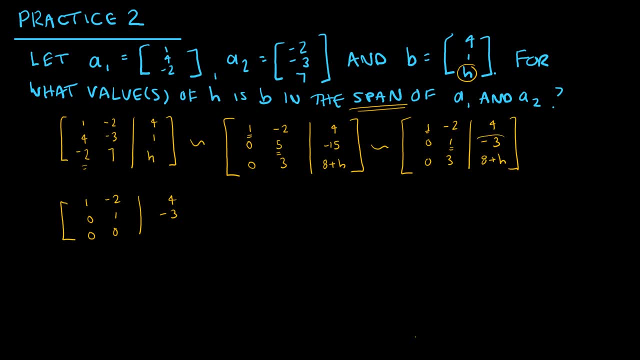 taking negative 3 times 3 negative 3, which is 9 plus 8, which is 17 plus H. now here's the problem: the only way to get the same number of rows is to take. the only way to get the same number of rows is to take the. 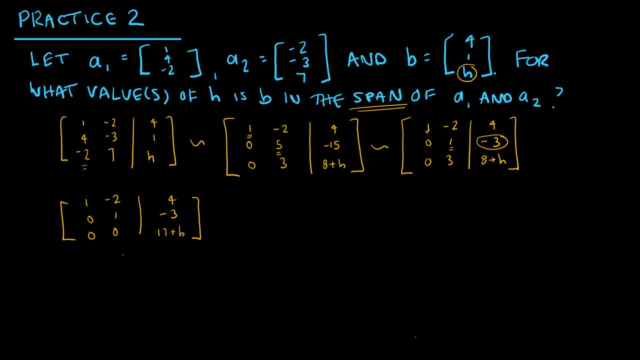 way that this works is if 0 equals 0 on this last row, because if H was some way that this works is if 0 equals 0 on this last row, because if H was some value that made it not 0, then this would not be valid. so, essentially what? 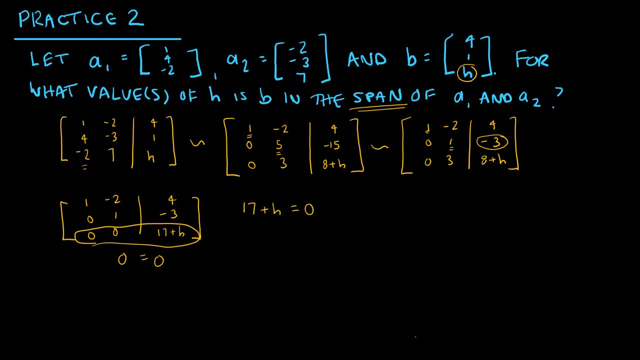 I'm saying is 17 plus H must be equal to 0, so H must be equal to negative 17. so the question is: what is the answer to the question is: what is the answer to the question is what value or values of H and H must be negative 17 for B to be in the span of?